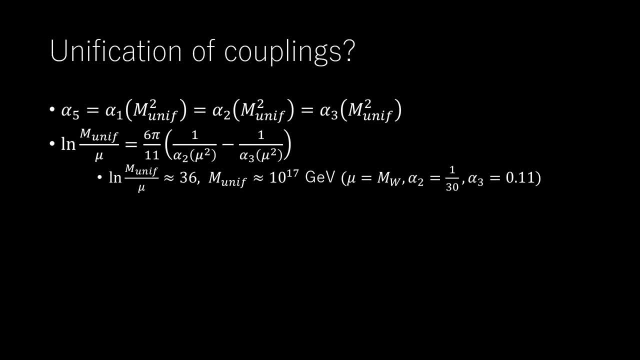 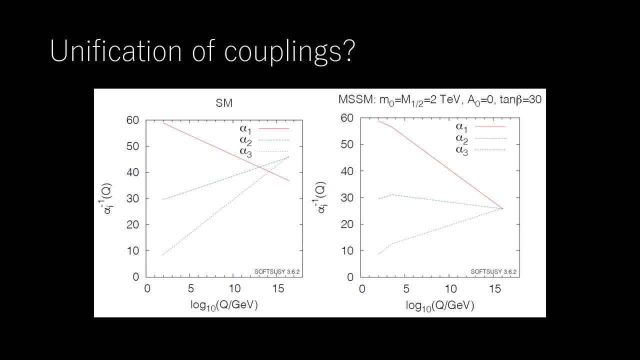 could the forces of particle physics finally have the same strength? Graphically, we have approximately the situation in figure, since each one over αi is a linear function of natural log of MUNIF over αi. This is the situation in figure, since each one over αi is a linear function of natural log of MUNIF over αi. 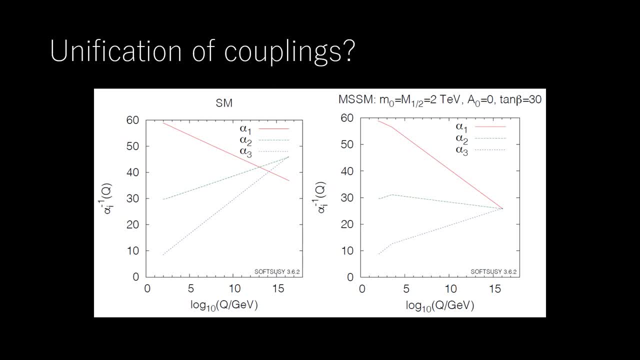 This is the situation in figure, since each one over αi is a linear function of natural log of MUNIF. over αi, The slopes are determined by the Bi, that is, by the gauge fields and the particular group structure. Given the values of the αi, 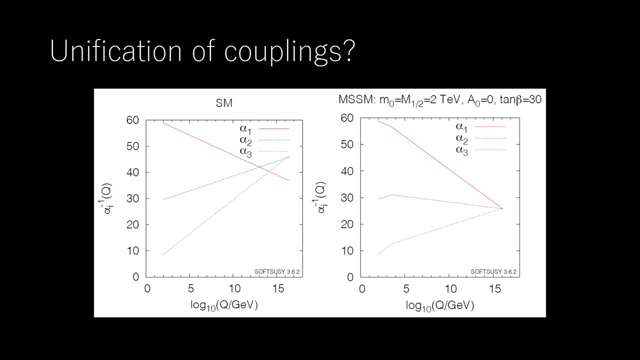 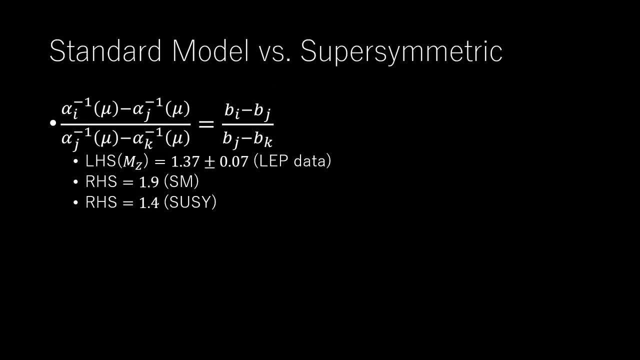 measured at, say, Mz and the slopes that are characteristic of the theory. we can calculate for any theory whether or not the forces unify. In some guts the couplings indeed meet at a point within the accuracy required by the measurements at Mz. for example, in a supersymmetric SU gut, In the super-symmetric SU gut. 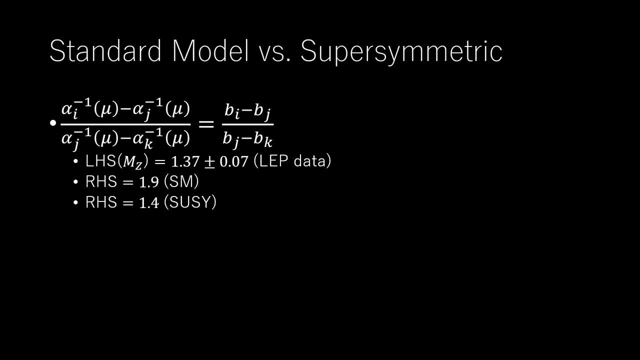 In the supersymmetric theory, the superpartners also enter the loops and change the coefficients somewhat. An interesting way to examine which theories give unification is to combine the running equations to give the following ratio: The left hand side can be evaluated from data. 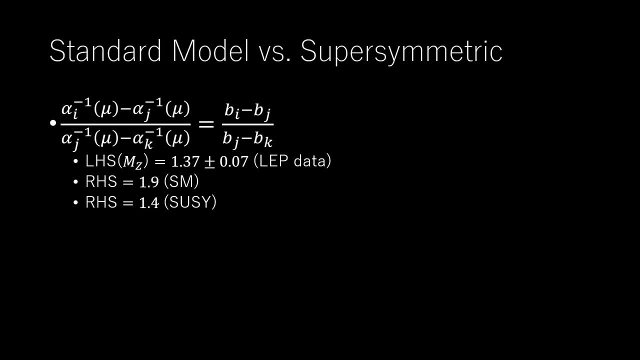 and the right hand side can be found from different theories. LEP data gives the left hand side, MZ equals 1.37 plus minus 0.07.. In the standard model, the, the right-hand side equals 1.90, so the unification is approximate When superpartners. 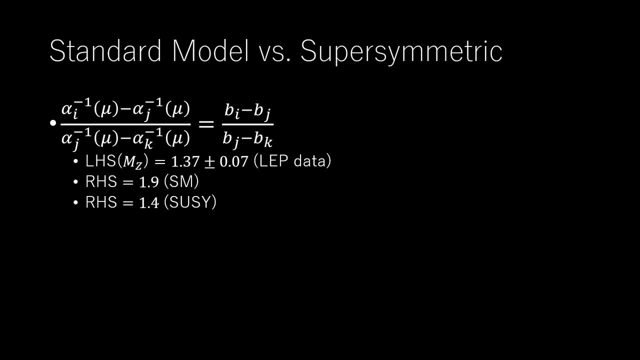 are included in the loops and there are two Higgs doublets as is necessary. in the supersymmetric extension. the right-hand side equals 1.4, which is consistent with the left-hand side given by the LEP data Within experimental errors. the supersymmetric extension of the standard model. 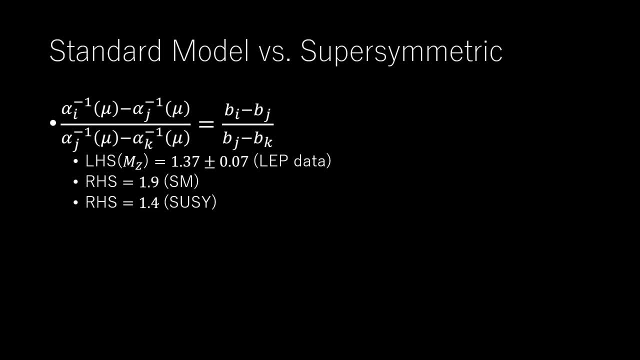 fully unifies. This is one of the reasons people have been enthusiastic about nature being supersymmetric.